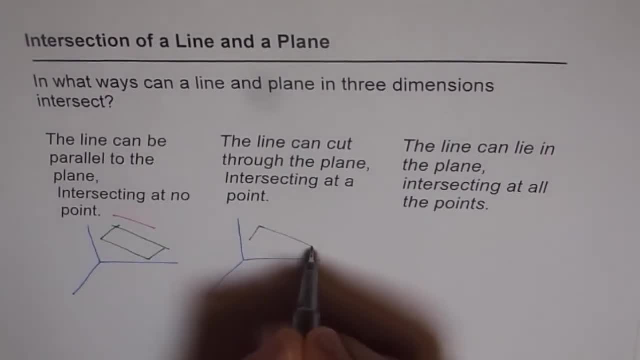 and let me sketch a plane again here, like a parallelogram right, Which looks more like a rectangle in this case- And let's say there is a line coming here So it intersects and just passes through the plane. Do you see that? So this line actually intersects at a point. So that is second case. 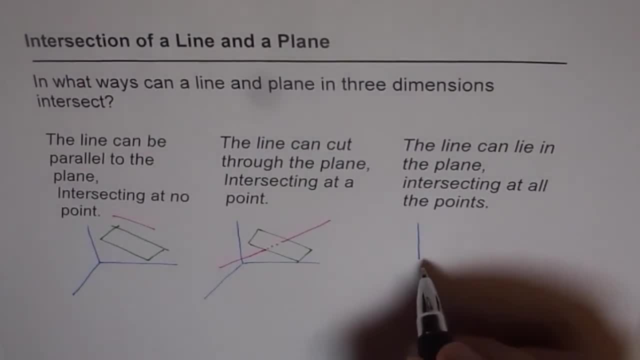 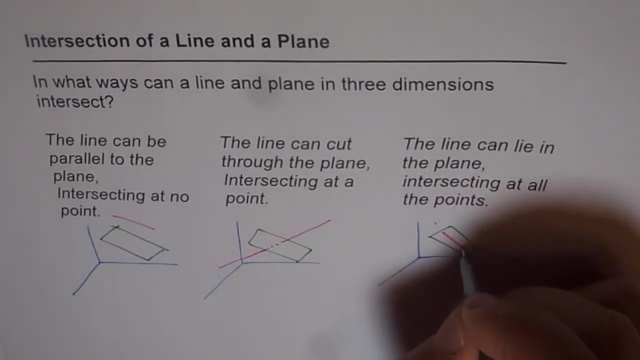 And the third case is that line could be contained in the plane itself, right? So the line could be in the plane. So that is the third case. So we have a plane here and the line is in the plane, Right Inside the plane itself. So these are the three conditions which we have when we 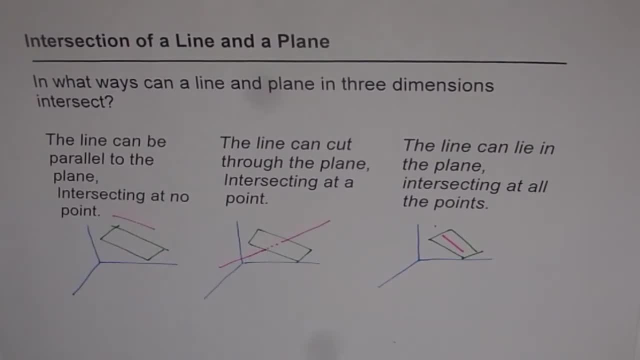 are considering line and a plane. So a system which consists of a line and a plane will have either no solution- will have one solution- or infinite number of solutions, right? So that is as far as the systems and solutions- systems solutions are concerned. Now, in this set of videos, we will see different cases and find out. 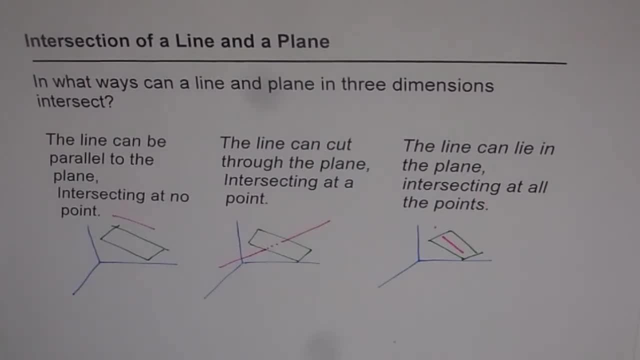 how lines and planes can intersect and what are their points of intersection. Also important thing to note here is that actually plane can also intersect. these are also lines, right coordinate axis, so planes can intersect with the coordinate axis, as you can see here right. So planes actually extend infinitely. so when you extend them they extend the coordinate axis. 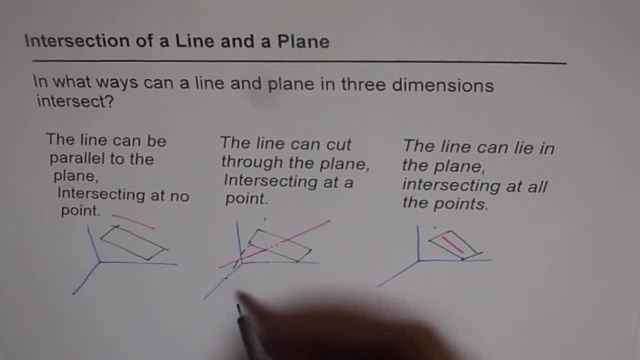 So those are their x, y and z intercepts Planes also intersect with the with x? y plane, y z plane and x? z plane, right. So we'll consider those cases also in this chapter and you'll also appreciate that sometimes it becomes helpful to find the point of intersection so that we 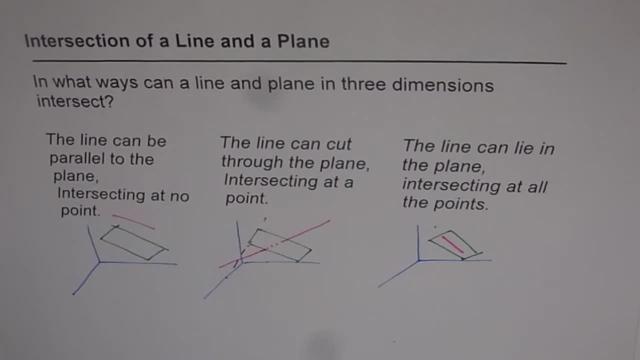 can actually find the point of intersection. So the other type of examples which you'll find in this set of videos is sketching planes, knowing their point of intersections. So let's explore more about lines and planes in these set of videos. Thank you and all the best.